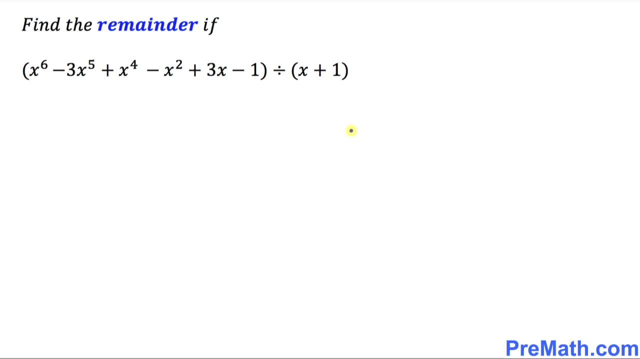 Welcome to pre-math. In this video tutorial we are going to find the remainder if this given polynomial is divided by x plus 1.. So the easiest possible method is called remainder theorem. So we're going to be using this one to find a remainder, and the remainder theorem has this: 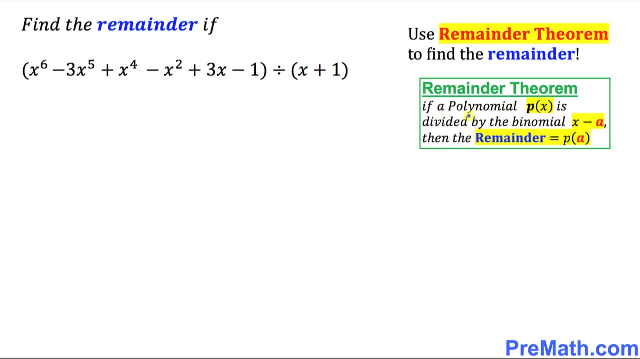 definition over it. It states: if a polynomial p of x is divided by the binomial x minus a, then the remainder is going to be equal to p of a. So let's get started now. The very first step is this one. Look at this one. This is called the dividend, isn't it? So this dividend I want to call. 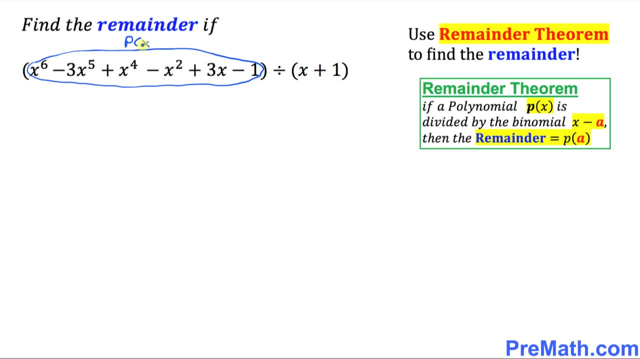 this one, p of x. P stands for polynomial, So I am going to write down p of x equal to this big long string. Okay, just put down: x power 6 minus 3x power 5 plus x power 4 minus x power 2 plus 3x minus 1.. And our next step is: 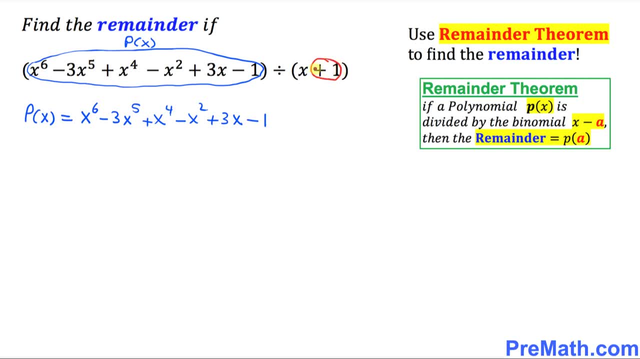 look at this divisor, this part, only positive. 1. The opposite of this one, the opposite sign, is going to be negative one, always, always, whatever this sign is, just put the opposite. so I'm going to go ahead. wherever I see X variable, replace it by this negative one. so our next step is going to be so this: 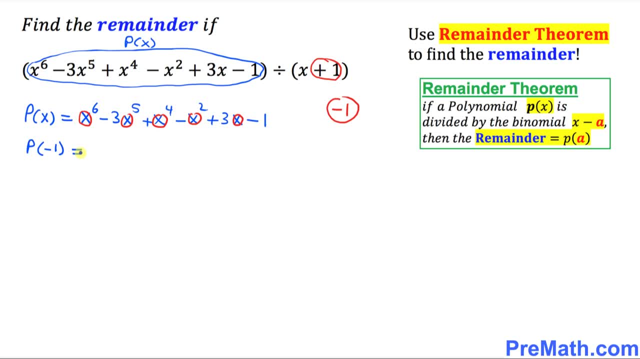 become P of negative 1 equals 2. so wherever you see X, replace it by negative 1. power 6 minus 3 times negative 1. power 5 plus negative 1. power 4 minus negative 1. square plus 3 times negative 1 minus 1. our next step: 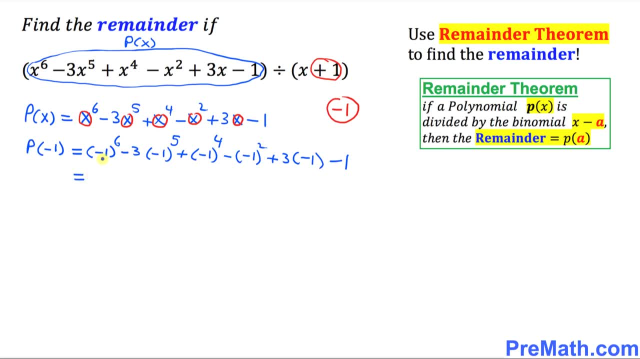 is just so. we are going to go ahead and do. the next step is just simplify. okay, that's all. so negative 1 power if you have an even power, so this become positive 1 minus 3 times when negative 1 has a odd power. that's going. 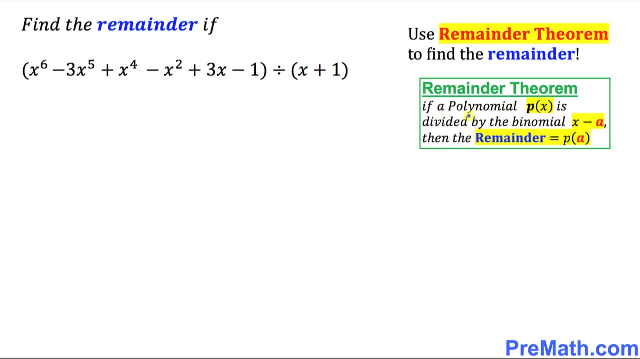 definition over it. It states: if a polynomial p of x is divided by the binomial x minus a, then the remainder is going to be equal to p of a. So let's get started now. The very first step is this one. Look at this one. This is called the dividend, isn't it? So this dividend I want to call. 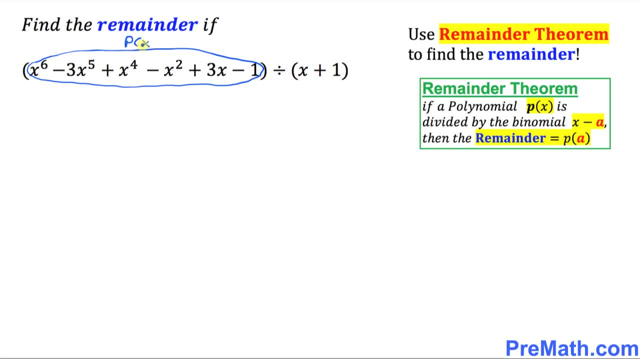 this one, p of x. P stands for polynomial, So I am going to write down p of x equal to this big long string. Okay, just put down: x power 6 minus 3x power 5 plus x power 4 minus x power 2 plus 3x minus 1.. And our next step is look at this divisor, this part only. 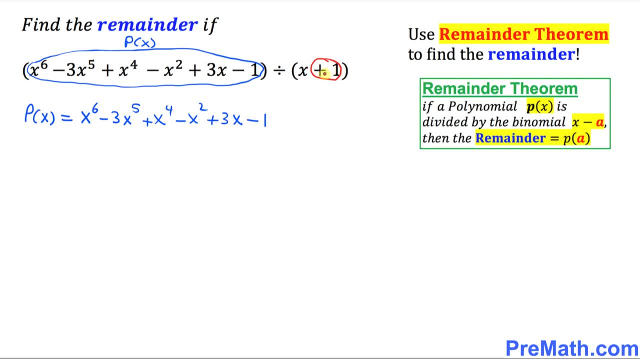 positive one. The opposite of this positive one is this one. So this one is going to be equal to one. the opposite sign is going to be negative one, always, always, whatever this sign is, just put the opposite. so I'm going to go ahead wherever I see X. 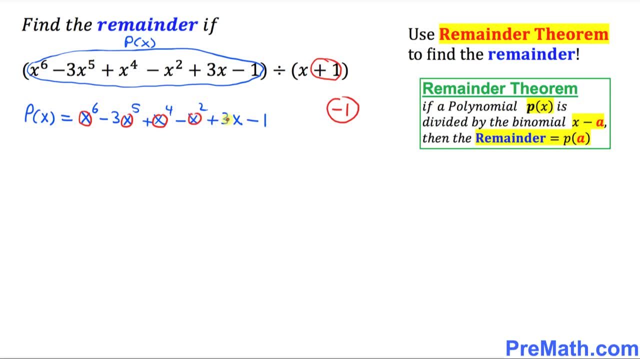 variable, replace it by this negative one. so our next step is going to be: so this become: P of negative 1 equals 2. so wherever you see X, replace it by negative 1. power 6 minus 3 times negative 1. power 5 plus negative 1. 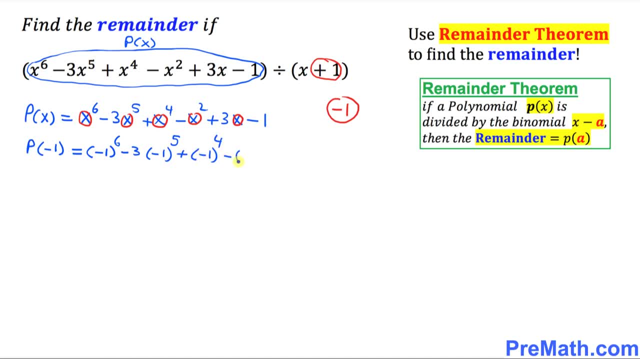 power: 4 minus negative, 1 square plus 3 times negative: 1 minus 1. our next step is just so we are going to go ahead and do. the next step is just simplify. okay, that's all. so negative 1 power if you have an even power. so this: 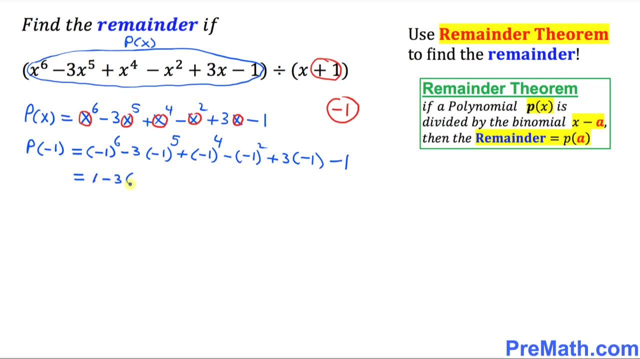 become positive 1 minus 3 times. when negative 1 has a odd power, that's going to give you negative 1 and over here, even power means this is going to be positive 1 and this is going to be a minus, and then this is going to be a.